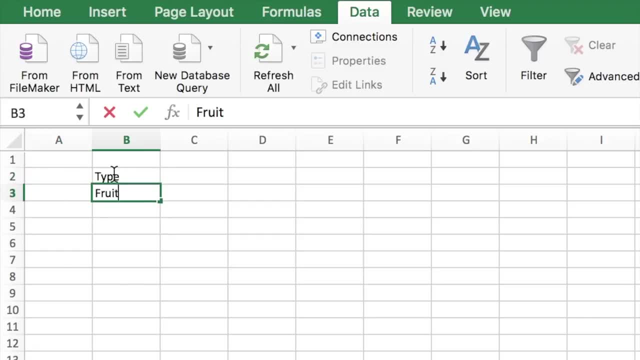 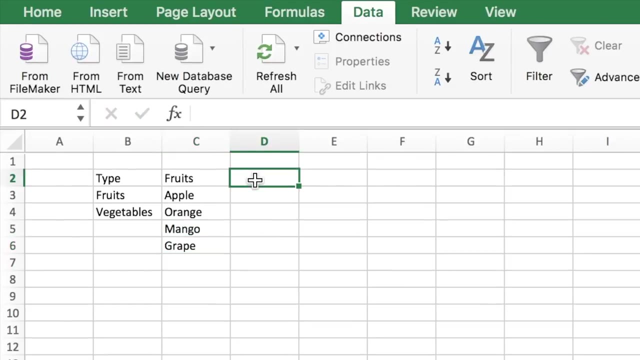 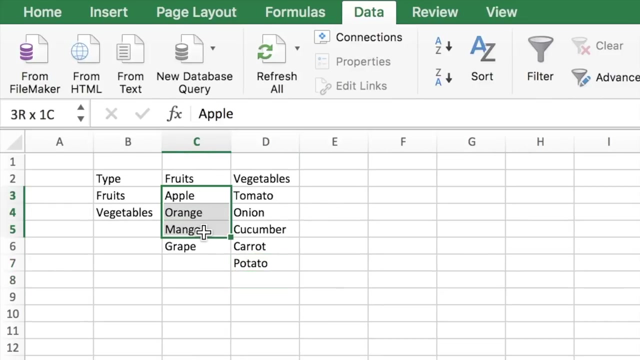 by first creating the type as fruits and vegetables, and to have the functionality of a dependent drop down list, you need to create the specific range. So let's begin with fruits and, similarly, vegetables. We need to now name the range which you created. 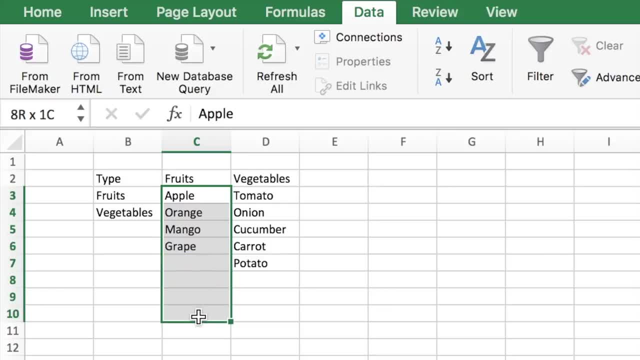 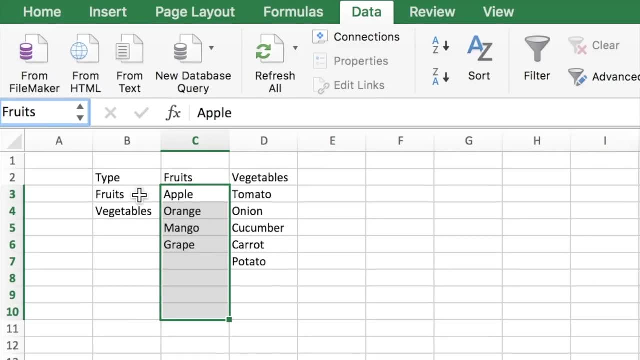 Okay, We could just select 4, but I would like to select extra in case you need to add more fruits later. And now you go to the top left corner and name this exactly as the type you have given as an option And just color it so that you know these are the amount of cells which form the range. 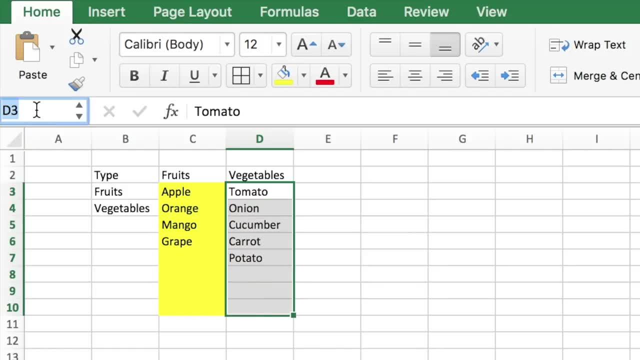 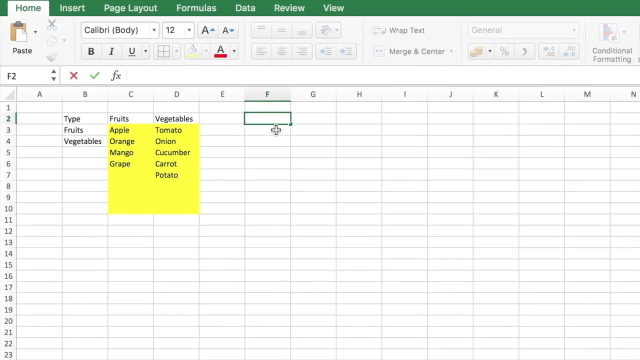 Similarly, you need to create for vegetables. So now, when you select this range of fruits, automatically, you know that this range is called fruits, which is same as the option in the type and similarly as vegetables. You are ready to go? Let's create a small table. 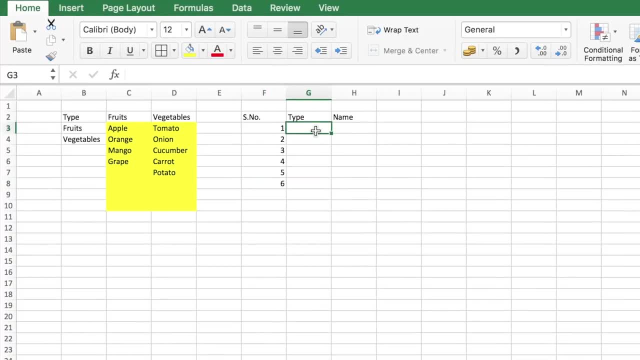 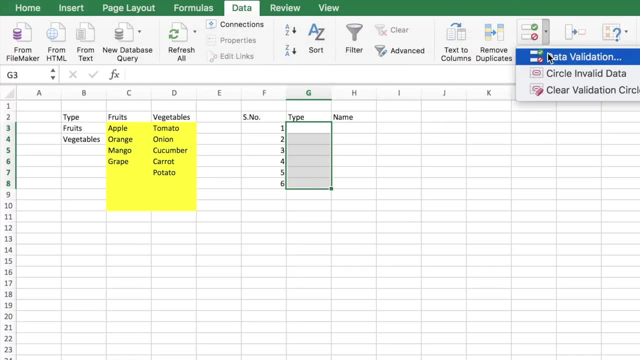 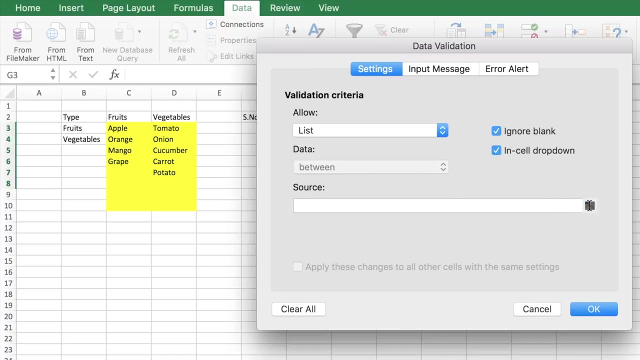 Now you need to use a function called data validation. So let's select the range and you go under the data tab: data validation. There, instead of allowing any value, you need to allow it to pick up from a list And the source as the fruits and vegetables option. 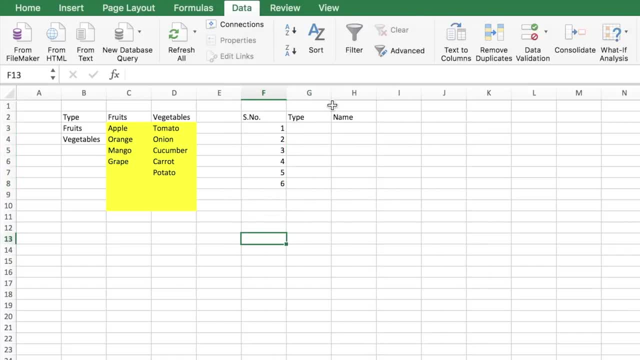 And you have an in-cell drop down. Okay, so now, when you go automatically, you have the option of fruits and vegetables. Now, with this, I would like to have a dependent drop down list. That is, if I select fruits, I would like to have a dependent drop down list. 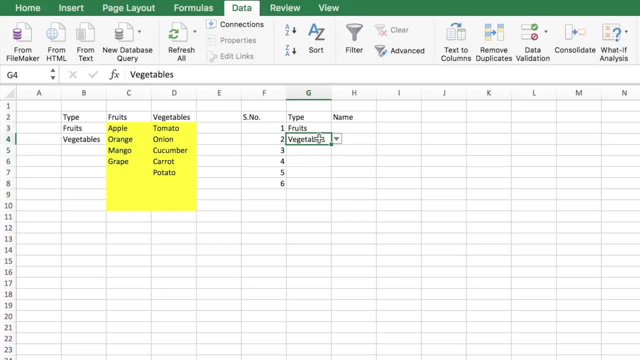 I would like to have the options which are in my fruits range And similarly, if I select vegetables, I would like to have the options in the vegetable range. This, again, can be achieved by data validation. Again, select the ranges. Go to data validation. 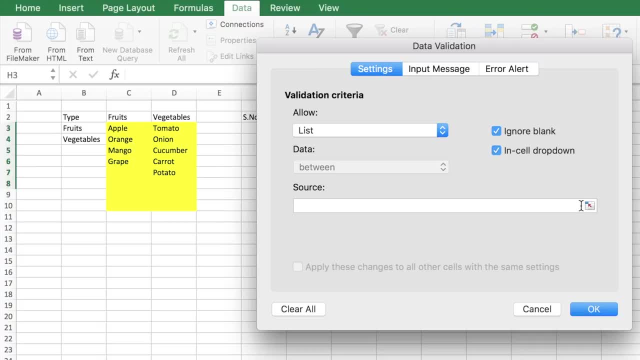 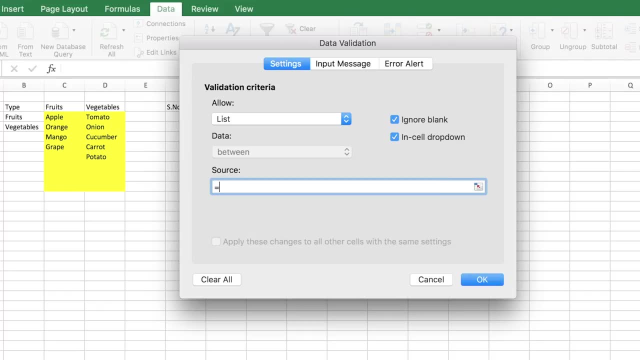 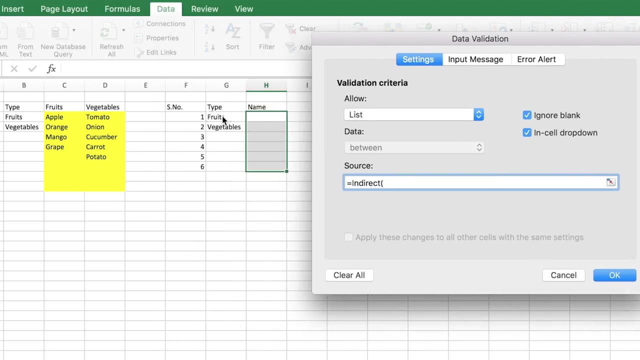 Instead of any value, it's going to be a list. Now we don't have a static source and it's going to be dynamic, depending on our initial option. So here you need to use a formula called indirect And select the cell value.